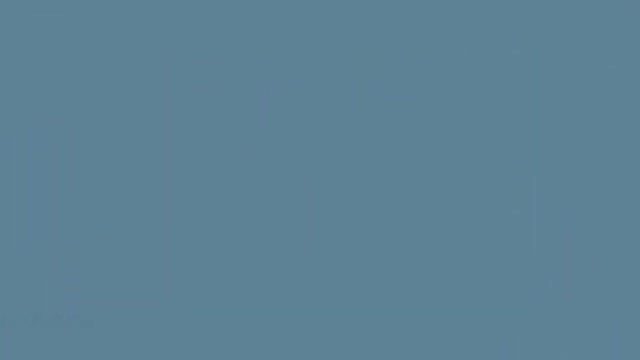 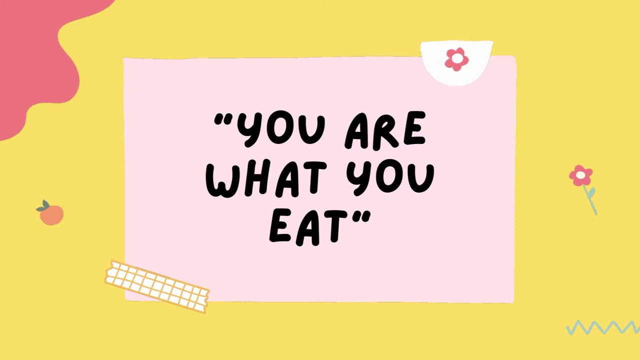 good outcome out of it. As the saying goes, you are what you eat. Good nutrition affects your total well-being. Thus, it is very important in attaining good health. As we go on to this topic, you will know that the health, of your health, is very important. So let's start with the 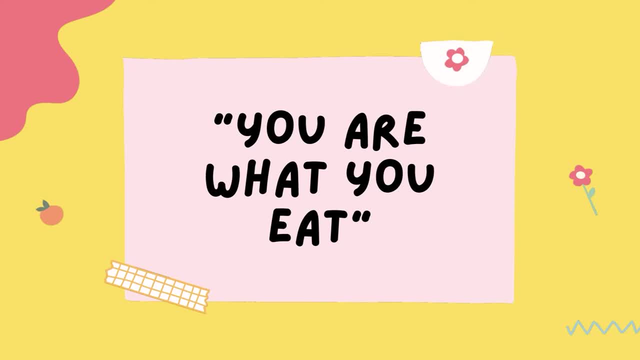 healthy food choices that are most important. How to eat well for good health is about how to make good food choices for a healthy, balanced diet throughout life. So what are the healthy foods for you? Healthy foods for you are the following. So for the healthy foods, you can include the following: You can include a healthy food from a healthy diet. There are many health benefits related to your diet. You can include an increase in dietary fiber, For example, a large amount of Studieng-Bacterial-B-B-B-B-B-B-B-B-B-B-B-B-B-B. These are all the health benefits that are affected by weight loss. However, if you have a healthy diet, you have to eat all the ingredients that are important. What kind of foods should you include? Health is an essential part of a healthy diet. 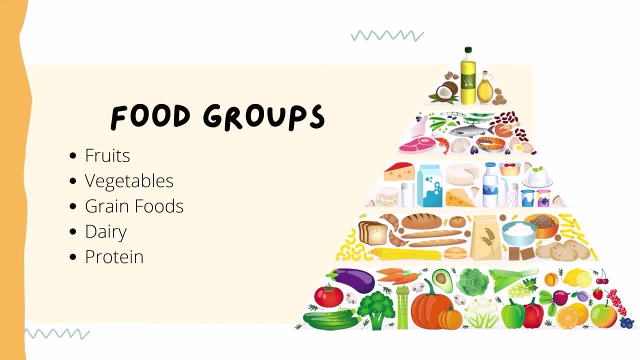 The health benefits are the most important ones. adolescent include a wide variety of fresh foods from the five food groups, which are fruits and vegetables, grain foods, dairy and protein. it's important for you to eat variety of foods from among these food groups. this will give you all the extra nutrition and energy you need to grow. 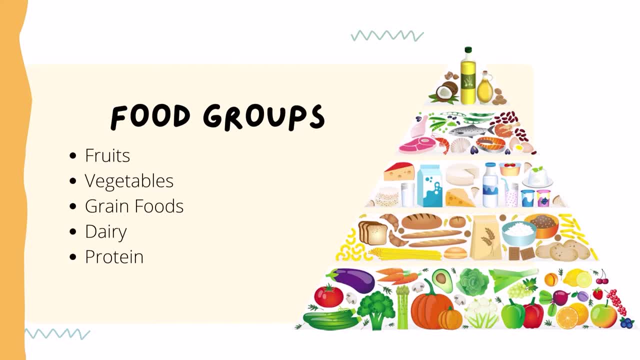 and develop properly. proper nutrition helps prevent diet related chronic diseases in the future, such as cardiovascular disease, cancer and osteoporosis. it is important for you to select a well-balanced diet. always remember that there is a strong relationship between what you eat and your health, not only today, but in the future as well. 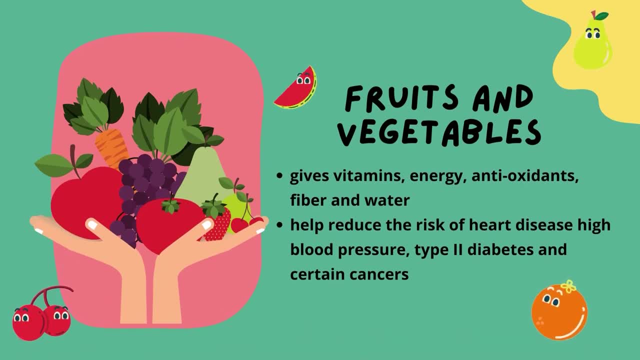 fruits and vegetables. fruits and vegetables gives you energy, vitamins, antioxidants, fiber and water. eating plenty of fruits and vegetables every day can help reduce your risk of heart disease, high blood pressure, type 2 diabetes and certain cancers. you should choose fruits and vegetables at every meal and for snacks to be in different colors, textures and taste, both fresh and cooked. 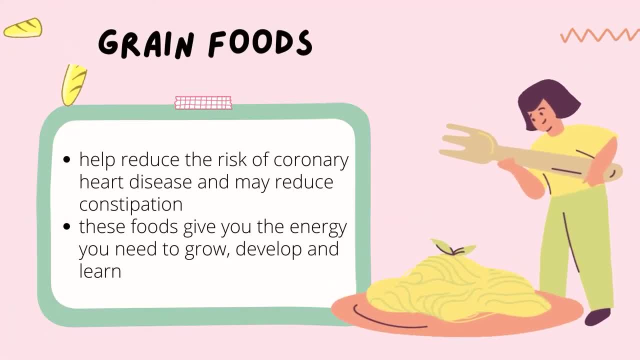 grain foods. consuming food rich in fiber, such as whole grains, as part of overall healthy eating reduces the risk of coronary heart disease and may reduce constipation. grain foods include bread, pasta, cereals, rice, corn and oats. these foods give you the energy you need to grow develop. 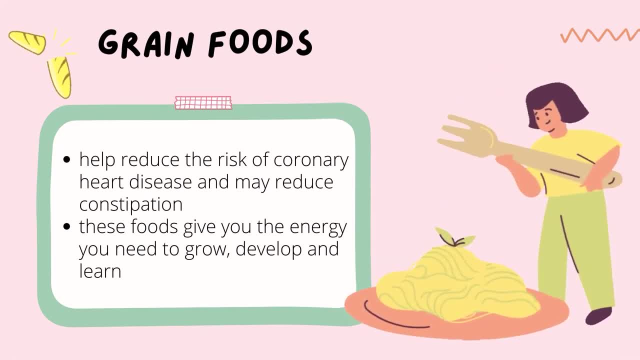 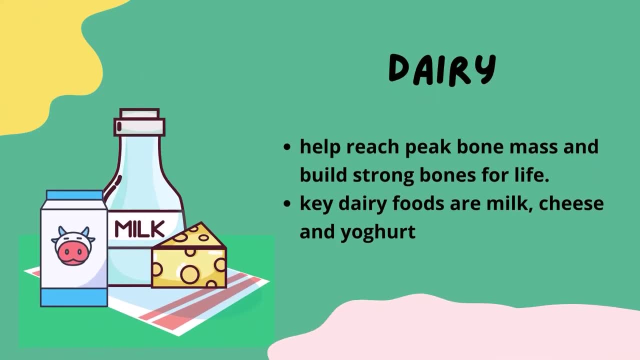 learn and will give you longer lasting energy and keep feeling fuller for longer dairy. during your puberty stage. you need more calcium to help reach peak bone mass and build strong bones for life, so you're encouraged to have different kinds of dairy each day. the key dairy foods are milk, cheese and yogurt. these foods are high in calcium and protein. 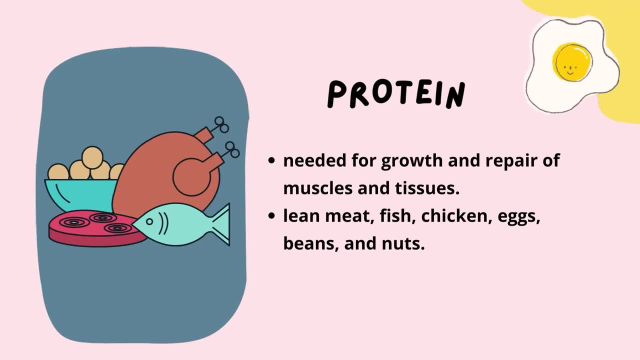 protein. protein is a hard-working nutrient. this needed for the growth and repair of muscles and tissues and the production of enzymes and hormones. these are especially important for an adolescent, as you experience rapid changes in development. in order for protein to do its job, you have to eat enough food to meet your daily energy needs. protein-rich foods include lean meat. 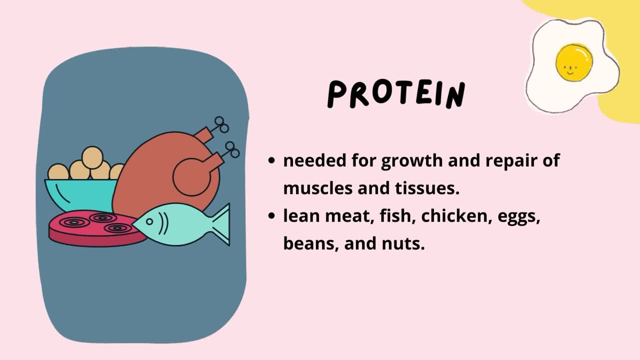 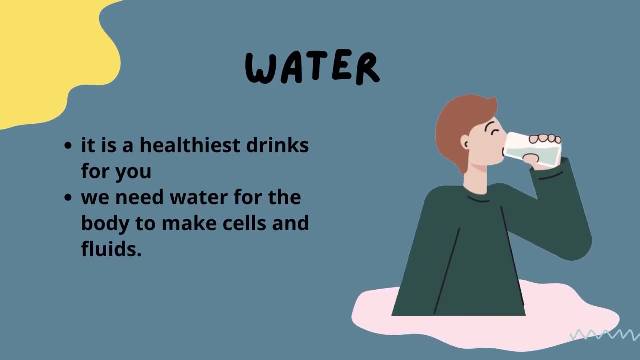 fish, chicken, eggs, beans, chickpeas, tofu and nuts. these foods are important for your child's development in growth of muscles, especially during puberty. what are the healthy drinks for adolescence? water. water is the healthiest drink for you. it is also the cheapest for mostら. we can live for about 18 months and more with how we eat. 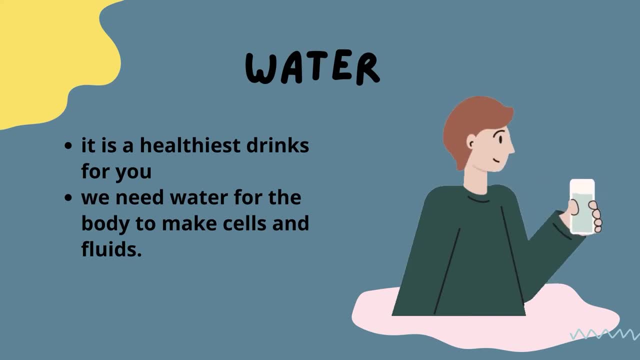 live without solid foods for weeks, but we cannot live without water for more than a few days. water is important for life. we need water for the body to make cells and fluids. it keeps mouth, intestines, eyelids and lungs healthy and wet for production of urine and sweat, to flush out waste from the body and other. 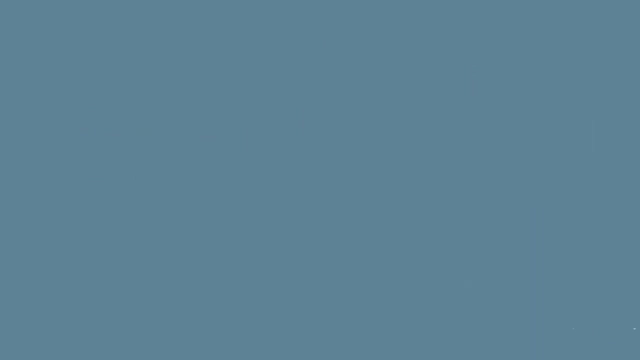 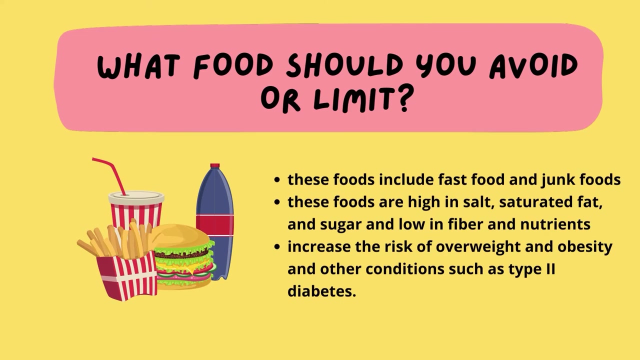 essential body processes. what food should you avoid or limit? you should mostly avoid. sometimes food or these foods includes fast food and junk food like potato chips, burgers, fries, pizza, cakes, chocolate candies, biscuits, donuts and pastries. these foods are high in salt, saturated fat and sugar and low in. 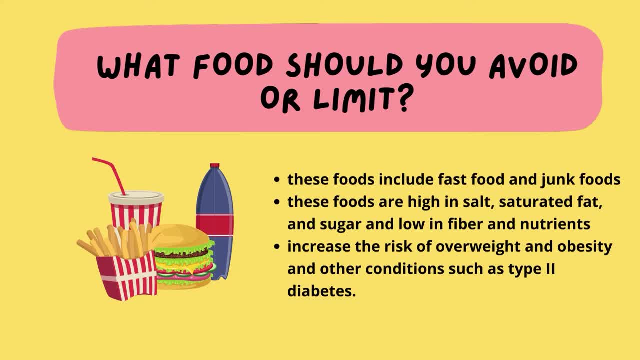 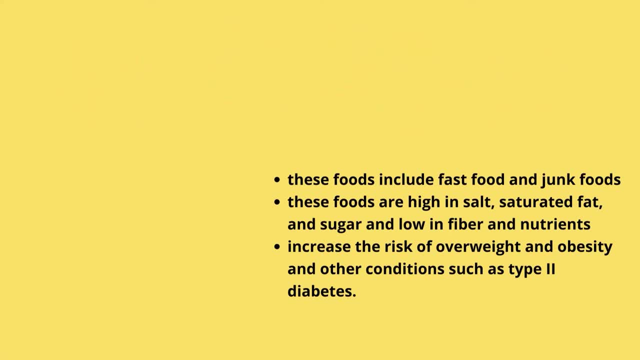 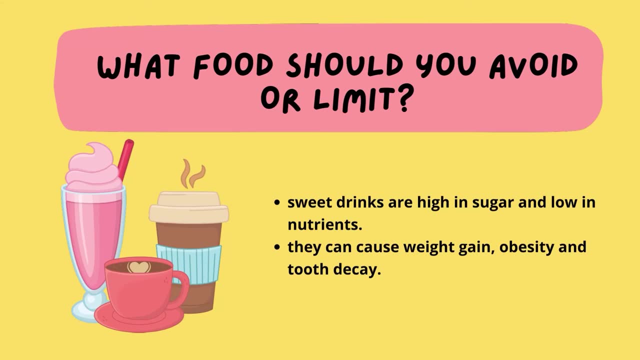 fiber and nutrients. too much of these foods can increase the risk of teenage overweight, obesity and conditions like type 2 diabetes. sweet drinks like fruit juice, sports drinks, flavored waters, soft drinks and flavored milk should take in small amount only. it cannot be avoided. sweet drinks are high in sugar and low in. 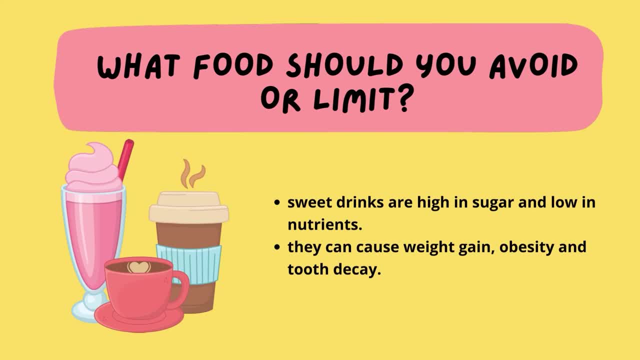 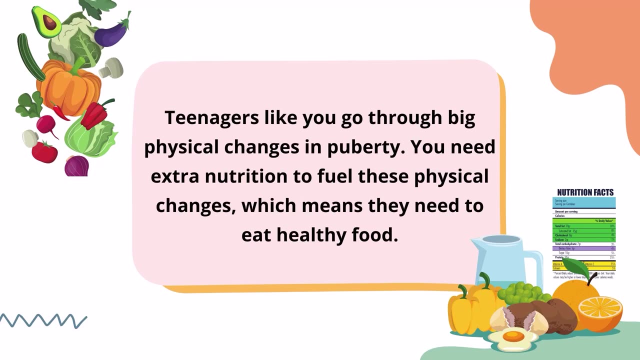 nutrients. they can cause weight gain, obesity and tooth decay. these drinks fill you up and make you less hungry for food and water for the rest of your life, for healthy meals. teenagers like you go through big physical changes in puberty. you need extra nutrition to fuel these physical changes, which means they need to eat. 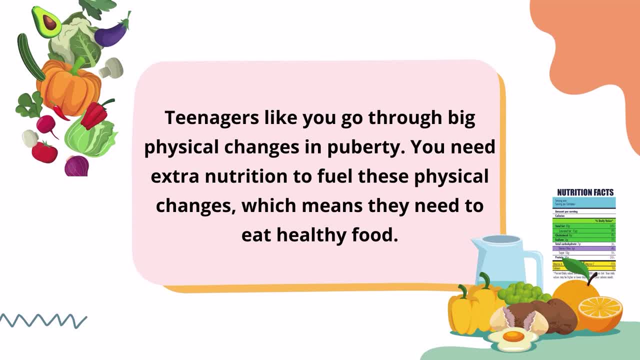 healthy food. your level of physical activity and stage of development will determine exactly how much healthy food you need. you'll notice you'll have bigger appetite, which is your body's way of telling you to eat more. remember what you eat a day will greatly reflect your health status in the future, to prevent the development of chronic disease later. 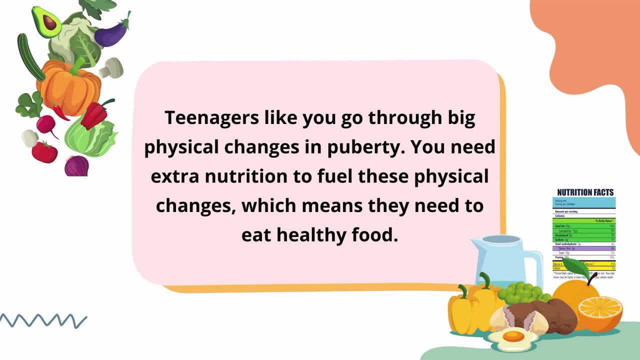 in life, it is important that you will always be careful in your food choices. that will be the end of our lesson one: all about food choices and how to eat well in your life. that will be the end of our lesson one: all about food choices, and stage of development will determine exactly how much you need to eat in your life. 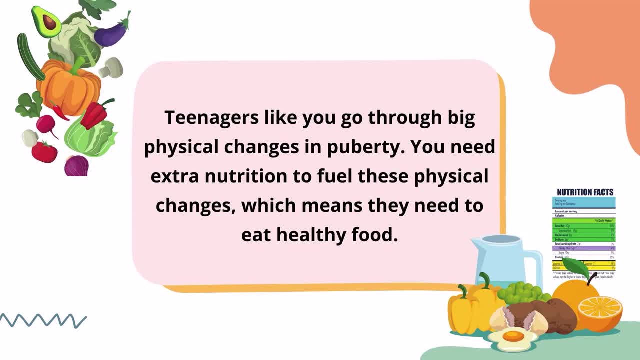 about nutrition for adolescent. thank you so much for listening and I hope you learned something. goodbye.